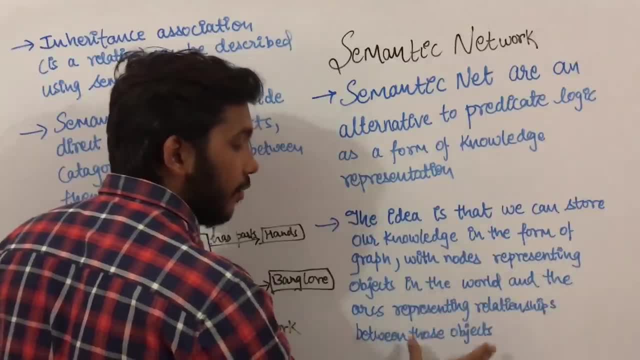 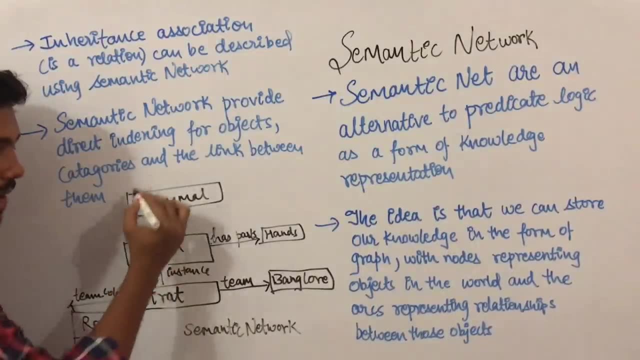 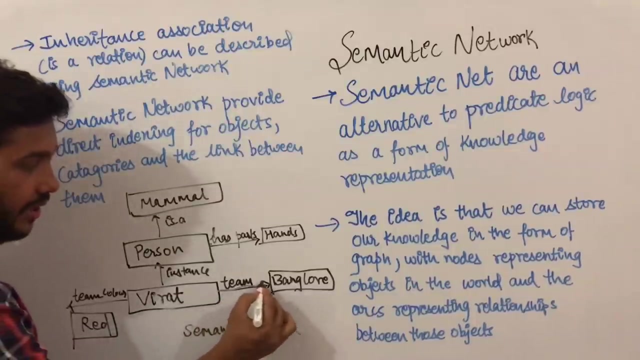 and the arcs representing relationship between those objects. Here Virat is an object, person is an object, Memal is an object, Bangalore is an object, hence is an object and red is an object. So we represent this real world object with the nodes, and now arcs represent. 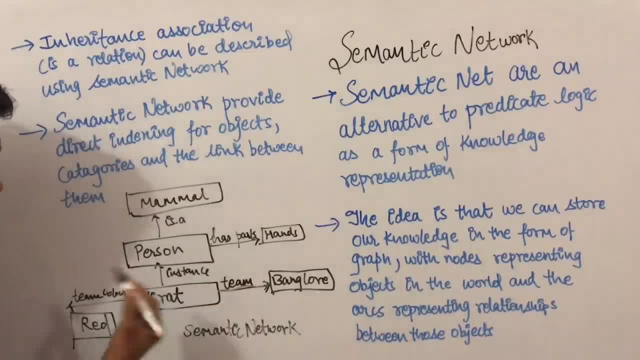 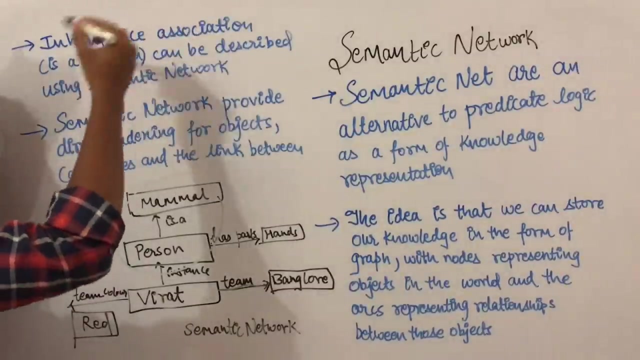 the relationship between the objects. like Virat is an object and Virat team is Bangalore, Virat team color is red. Virat is an instance that he is a person. person is another object. person has part, hence person is a Memal. This is an inheritance that person is a Memal, Inheritance association. 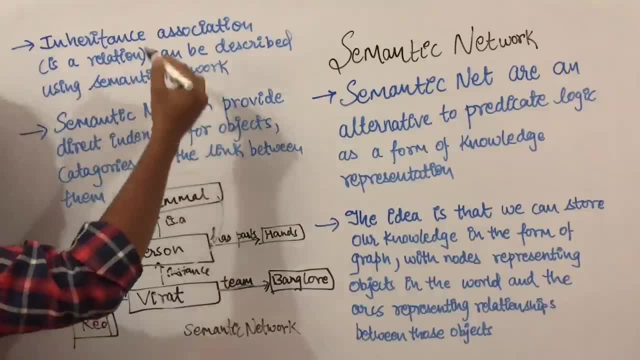 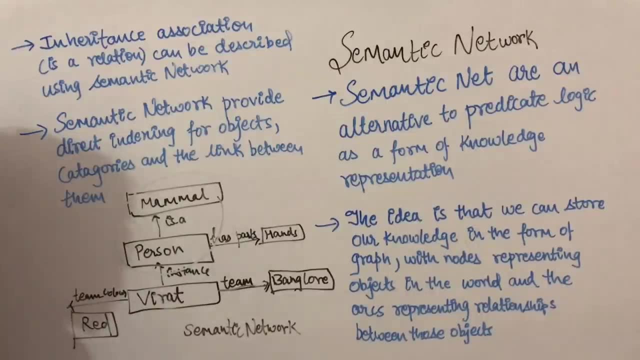 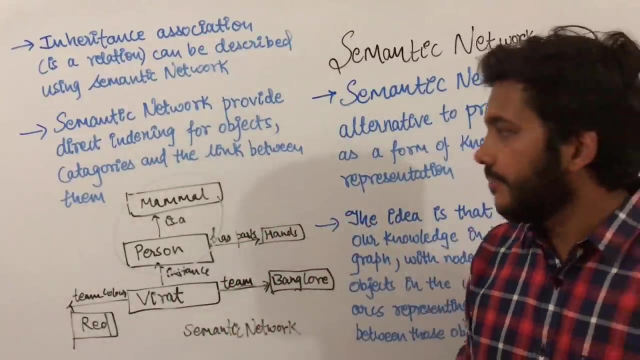 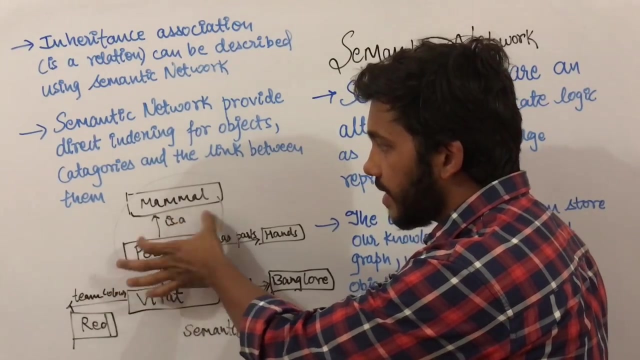 is a relationship can be described using semantic network. Representing inheritance in predicate logic was tough, But now representing this ISA relationship in semantic network is quite easy. We can represent one object like person and with the help of the relationship ISA, we can represent the inheritance association Semantic network. 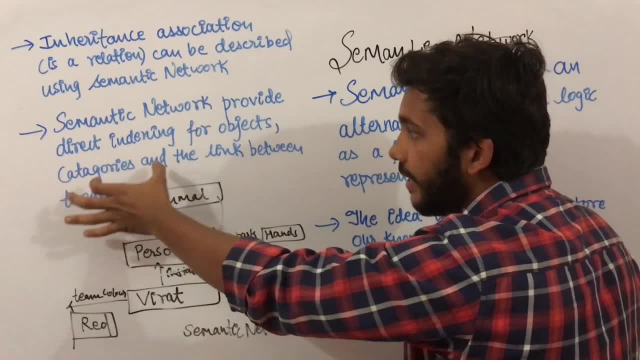 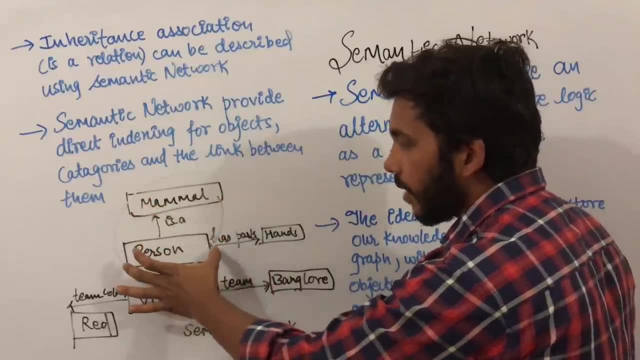 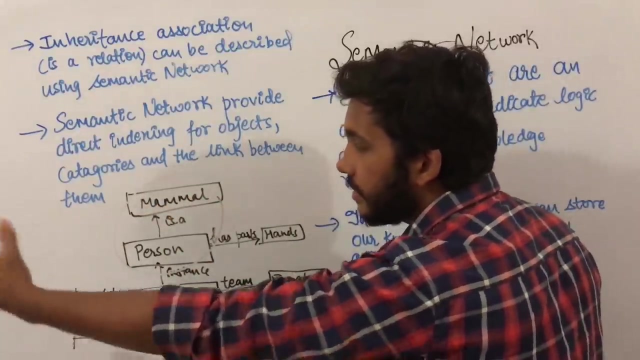 provide direct indexing for objects and categories and the links between the objects, For example between them. like we can category that mammal has persons and person can be virat, we can also categorize that mammal have animals, animals can be dog. so we can categorize the objects. 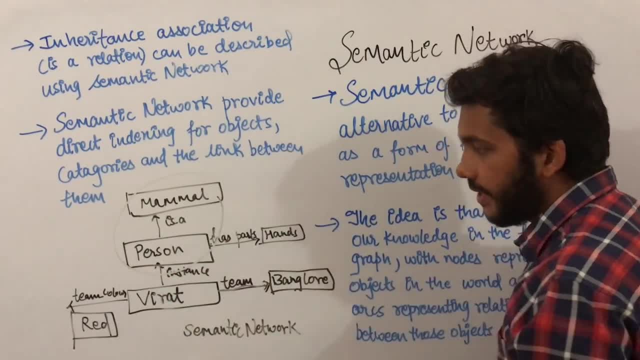 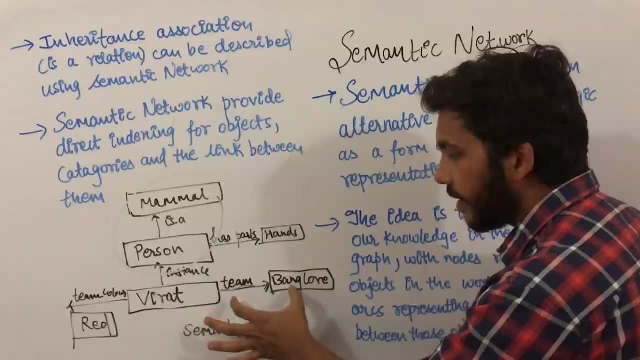 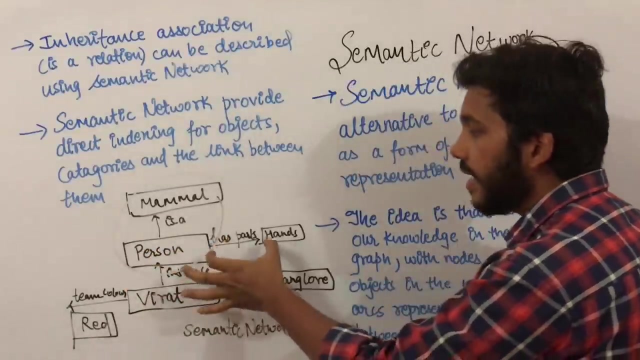 in different, different categories and now we can link between them. this is an example of semantic network. virat is of the team band load. virat team color is red. virat instance is a person. person has parts called hands. we can have different, different uh pro attributes of person. 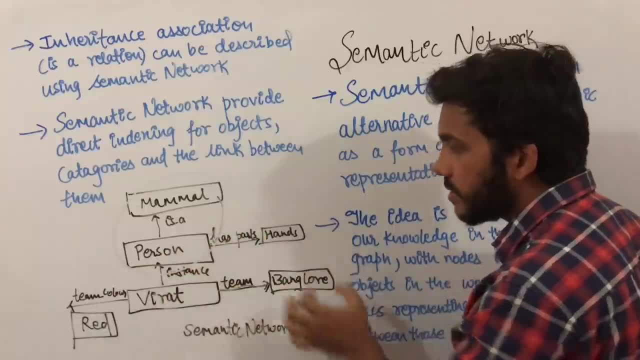 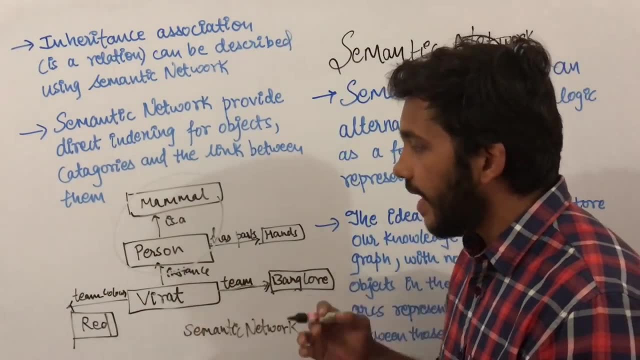 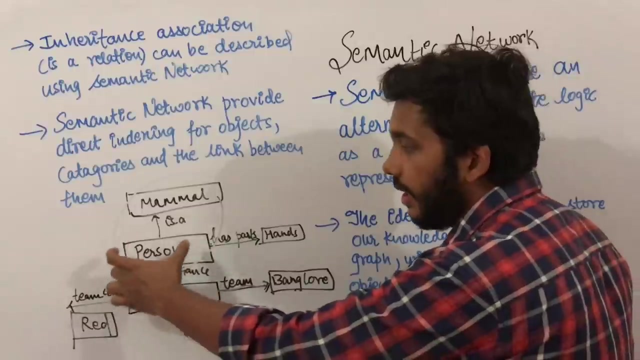 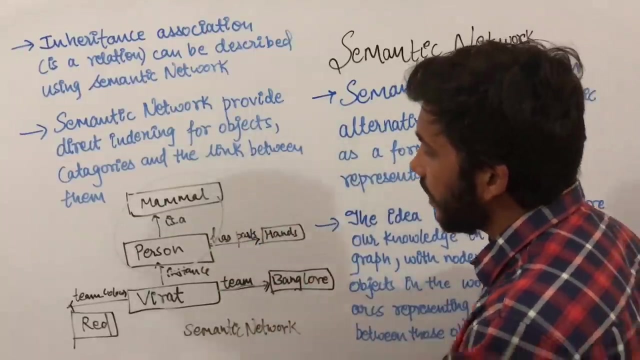 like one of the attribute for the person is: has parts we can on our. we can have another attribute: that person can see, person can smell, person has height, sex. so for our object we can have different, different attributes and we can depend, represent this different, different attributes with help of different nodes and we can represent the 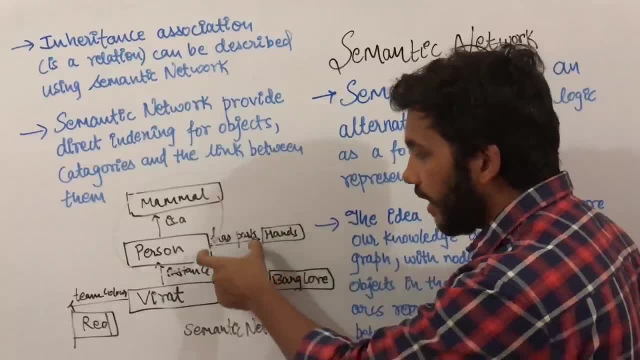 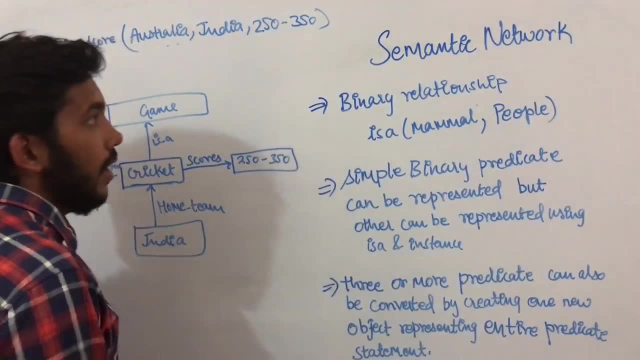 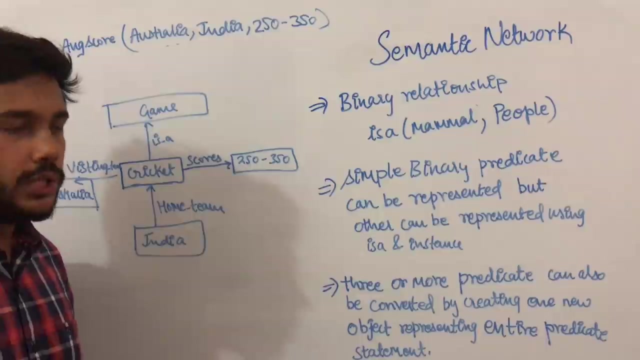 relationship between the nodes with the help of arcs, and this arcs represents the relationship between the different different nodes. now, coming to the binary relationship. binary relationship in predicate logic: what- is value? Почему? Late Party Reality, Orientation상. primary relationship- binary relationship in predicate logika, we note going to학. 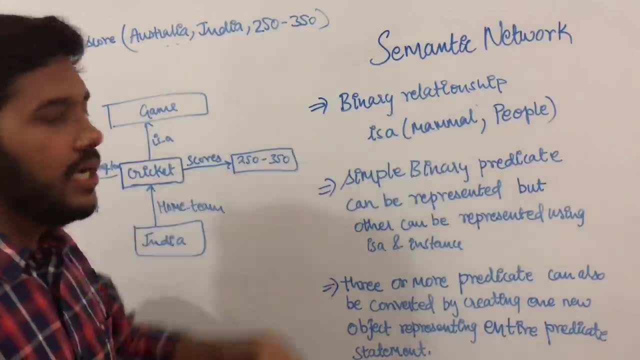 Teacher subject under some of the authors, that the setting of the favorite model, the formatting method, 삼 이거 bars in nosso. so yeh uichaa, uichaa. We are using allegors across management easy to represent. and now representing this binary relationship in semantic. 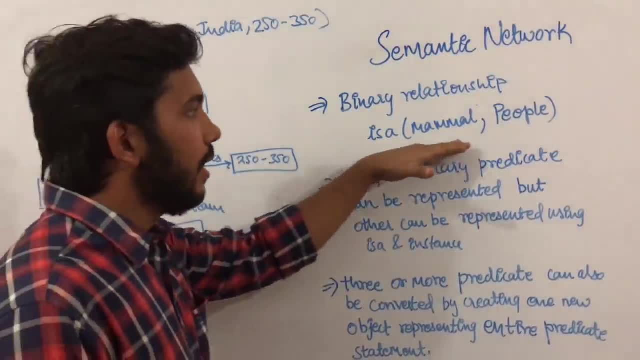 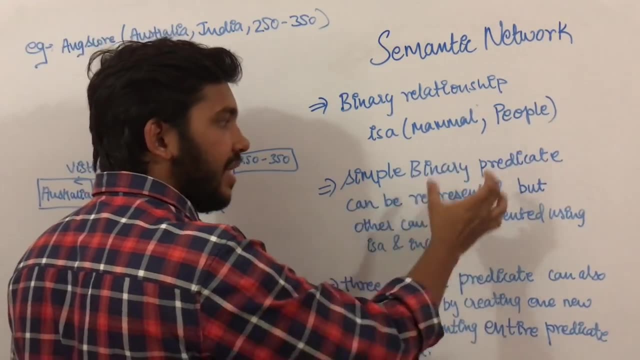 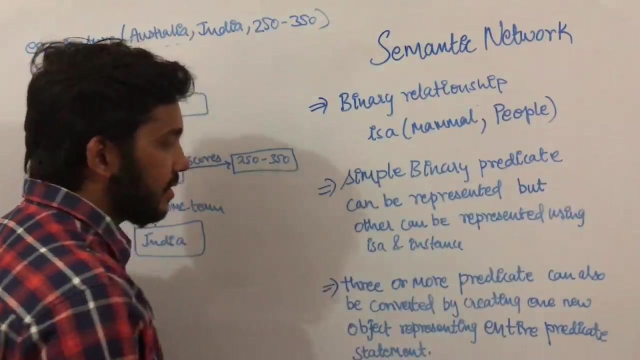 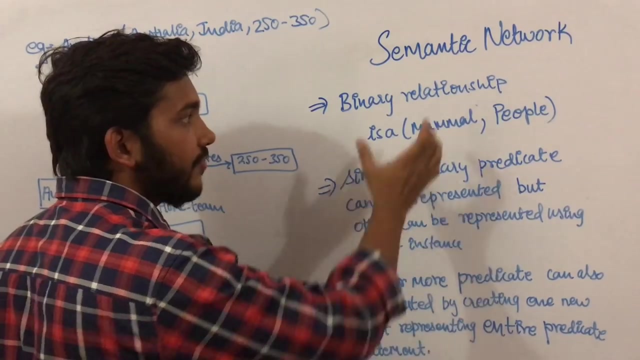 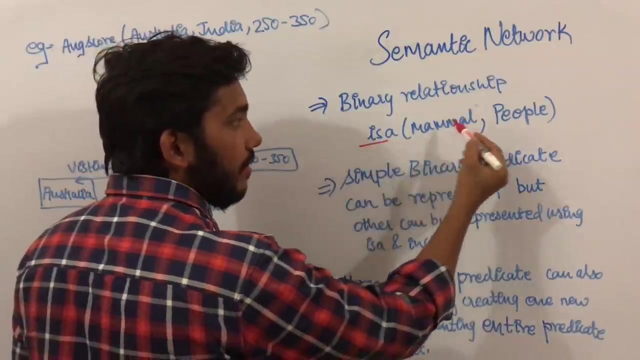 network is also easy because we can represent this binary relationship with is our relationship. simple binary predicate can be represented, but other can be representing, represented using is our and instance. if we have just simple binary size, simple binary relationship or simple binary inheritance relationship, then we can easily represent it with using is our and in bracket we can write: 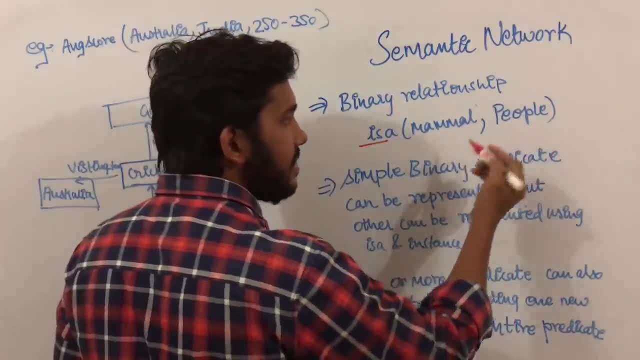 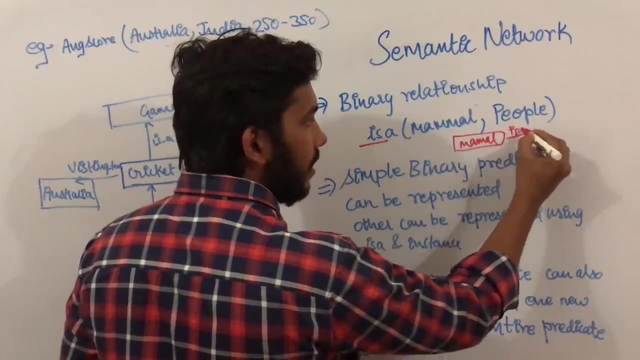 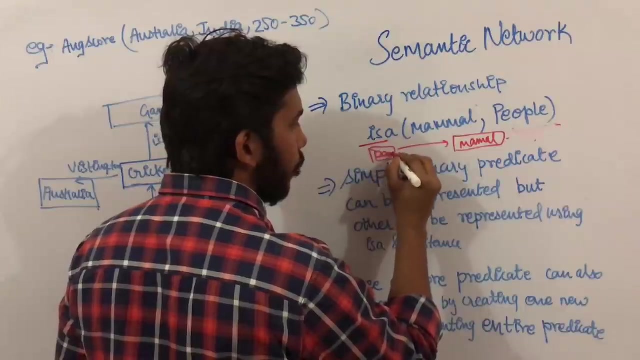 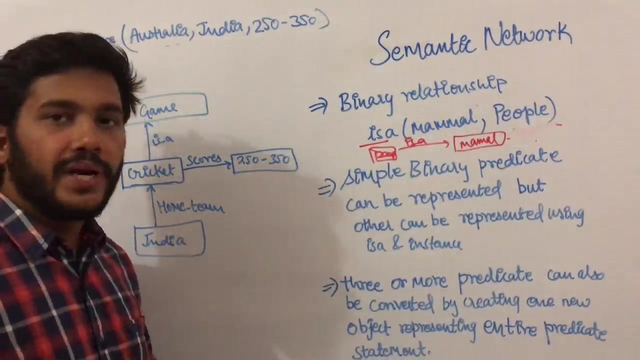 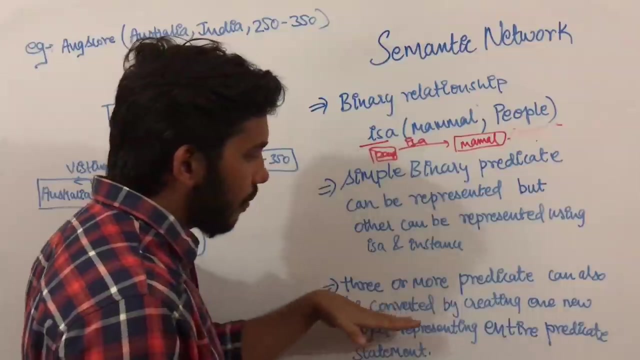 mammal comma, people, and this we can represent in semantic network as mammal is our, or you can say pupil is our mammal. if we want to represent three or more predicate relationship, then what we are going to do for three or more predicate we can also be converted. 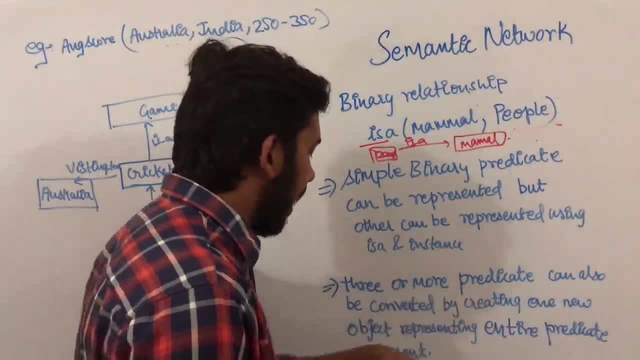 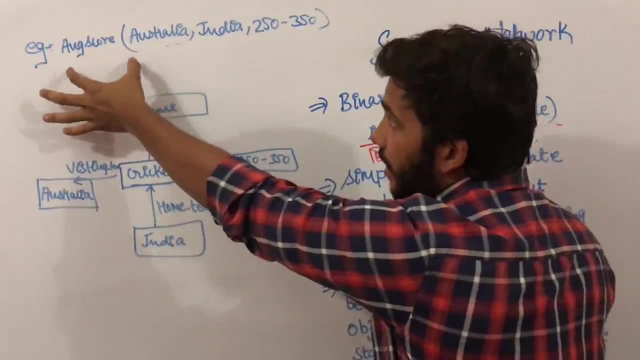 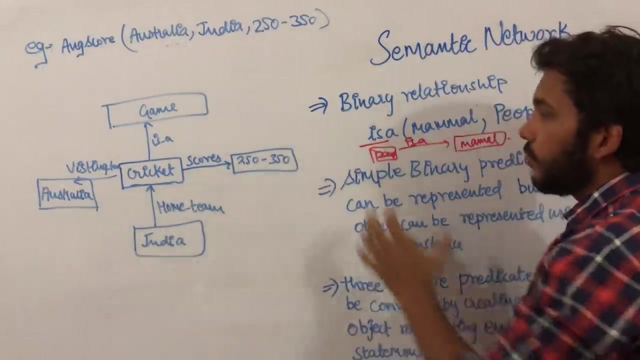 by creating one new object representing entire predicate statement. suppose this was our statement. average score- Australia, India- is 350 to 50 to 350, is 350 to 50 to 350. so this is not a simple binary relationship. this isn't in a three-form.